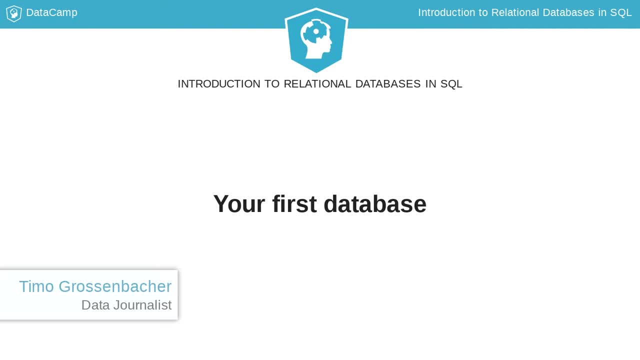 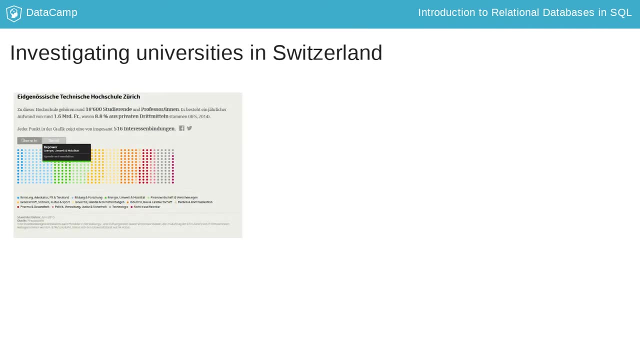 You'll learn how to create such databases and bring in to force their most prominent features. Let me tell you a little story first. As a data journalist, I try to uncover corruption, misconduct and other newsworthy stuff with data. A couple of years ago, I researched secondary employment of Swiss university professors. 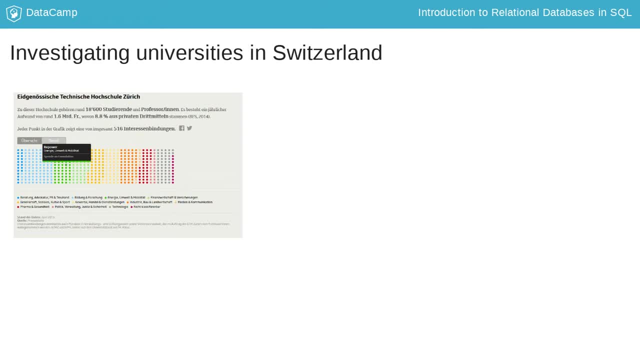 It turns out, a lot of them have more than one side job besides their university duty, being paid by big companies like banks and insurances. So I discovered more than 1,500 external employments and visualized them in an interactive graphic shown on the left. 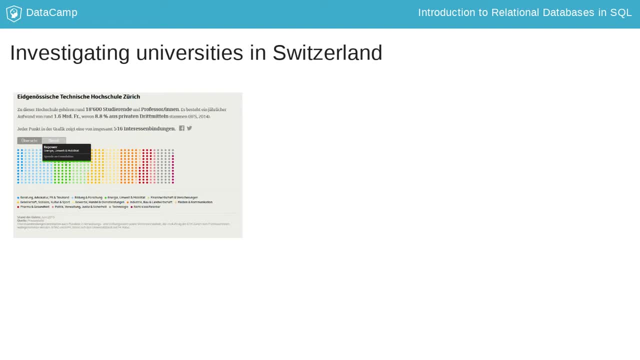 For this story, I had to compile data from various sources with varying quality. Also, I had to account for certain specialities, for example, that a professor can work for different universities or that a third-party company can have multiple professors working for them. 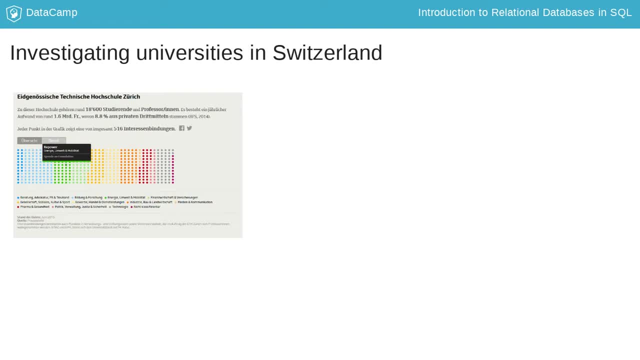 In order to analyze the data, I needed to make sure its quality was good and stayed good throughout the process. That's why I stored my data in a database whose quite complex design you can see in the right graphic. All these rectangles were turned into database tables. 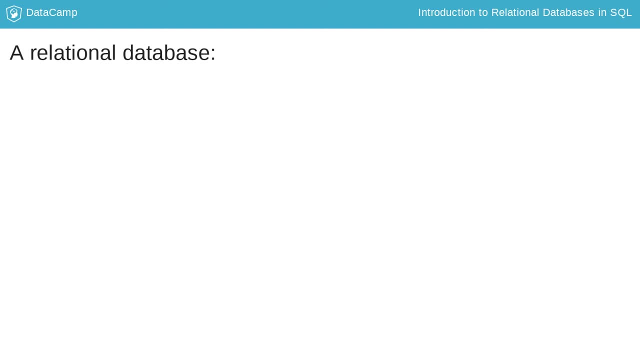 But why did I use a database? A database models real-life entities like professors and universities, by storing them in tables. Each table only contains data from a single entity type. This reduces redundancy. by storing entities only in tables, For example, there only needs to be one row of data containing the details of a certain company. 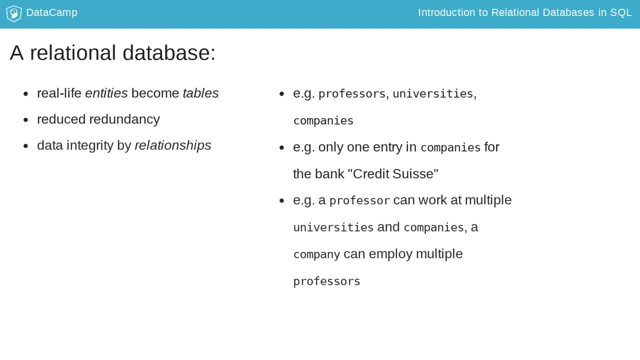 Lastly, a database can be used to model relationships between entities. You can define exactly how entities relate to each other. For instance, a professor can work at multiple universities and companies, while a company can employ more than one professor. Throughout this course, 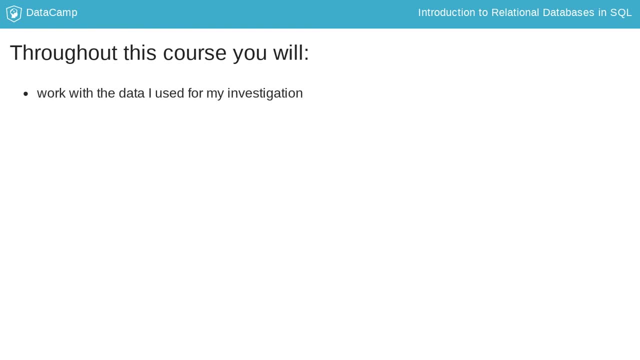 you will actually work with the same real-life data used during my investigation. You'll start from a single table of data and build a full-blown relational database from it, column by column, table by table. By doing so, you'll get to know constraints, keys and referential integrity.